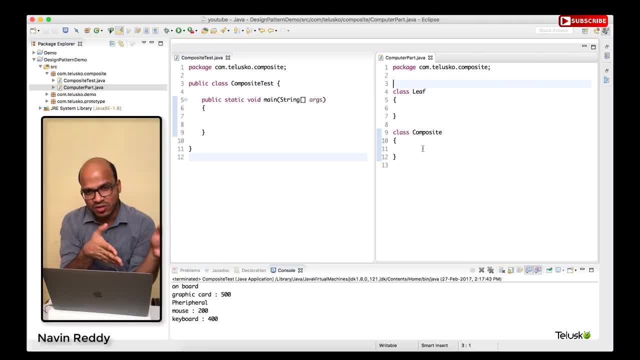 We have motherboard, we have hard drive, but inside hard drive also, in fact, motherboard also. we have two things: We have RAM and we have CPU, right? So when you have this structure, when you have this hierarchy, that if you want to talk about RAM it is inside a computer, 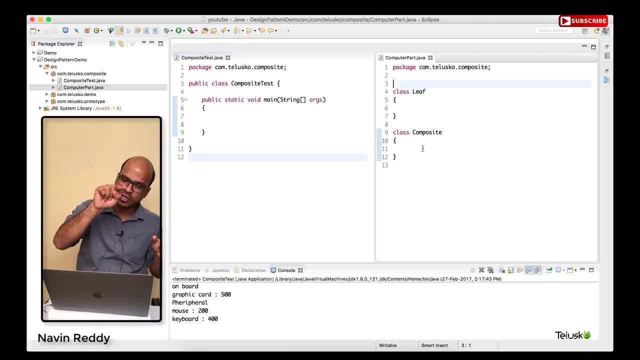 Inside the computer we have specifically inside your cabinet. Inside your cabinet it is specifically on your motherboard, and inside motherboard we have RAM. It goes in that sequence. So when you talk about the component, if you have a subpart of it- example cabinet- has a motherboard. 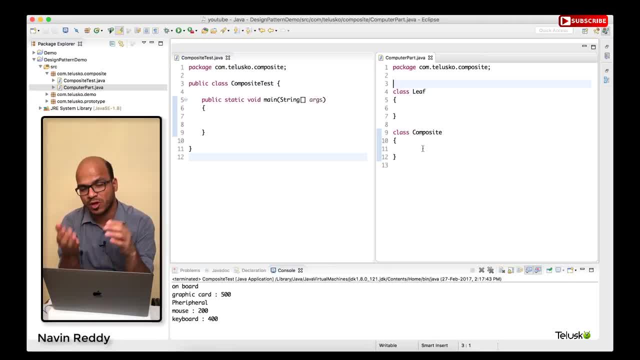 So cabinet will be called as a composite object because it has something inside it. But let's say, if you talk about the hard drive, we don't have anything inside the hard drive, right? It is called as leaf node Just to explain this concept. we have this code where I have a class which is composite, test, which has a main method. 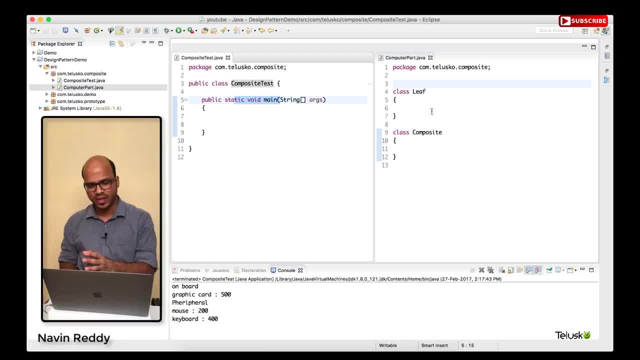 And then we have another class here, Which I mean another file, which is computer part, which has two classes: One is leaf and second is composite. So what I will be having inside leaf- example of leaf- would be hard drive, It will be RAM, CPU and all those things. 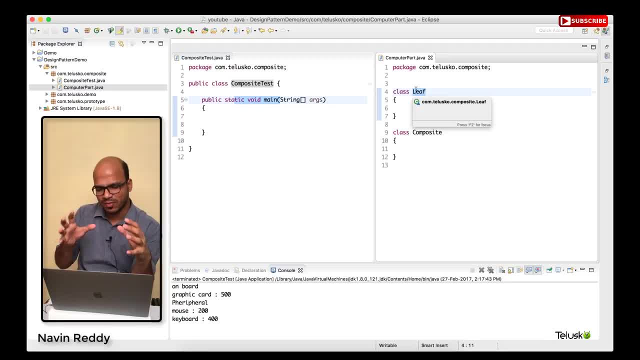 We will be not going for all the objects inside a computer, but some of them. So to achieve this, what we need here is so the main thing is here. If I ask you the price of a RAM, you have to be very specific. 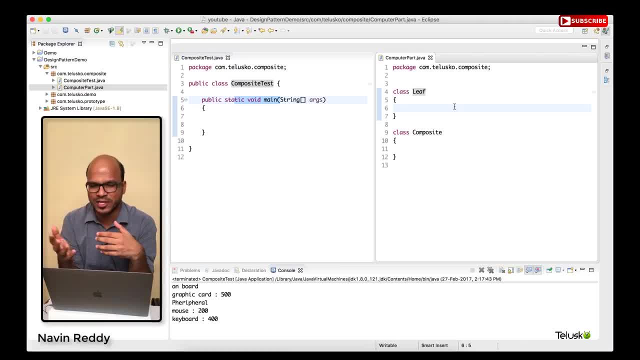 RAM will cost you around 2000 rupees. You can convert that into dollars, but let's say it is 2000 rupees. Or when you talk about a keyboard, it will cost you around 500 rupees. So we have certain cost for each object, right. 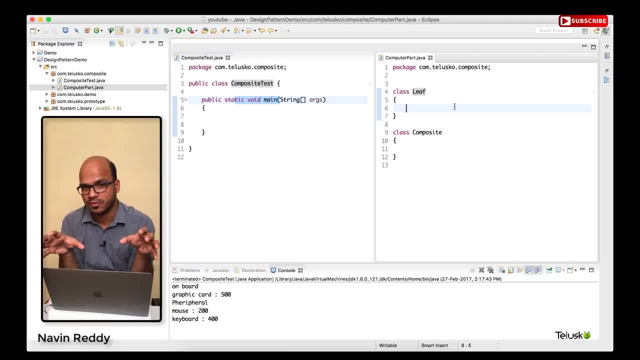 And whatever object I am talking about now, they are leaf object, right, But then if I ask you, what is the price of peripheral devices? Now, when I say, show me the price of peripheral device, you should be able to do that, Because whatever you can do with the leaf object, the same thing should be possible with the help of RAM. 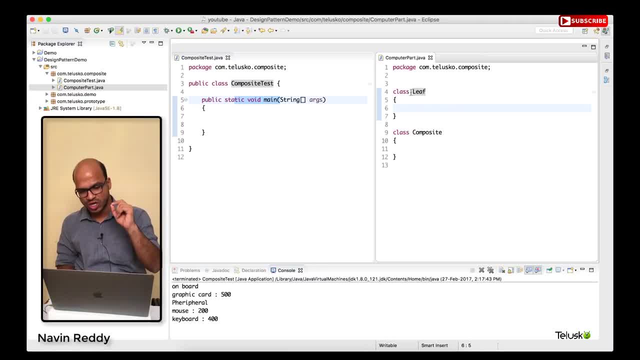 If you have composite object, that means this leaf and composite need to share some common feature. Now, both these are a component, right? So I will say I will create an interface here So that we will get some common thing between these two. 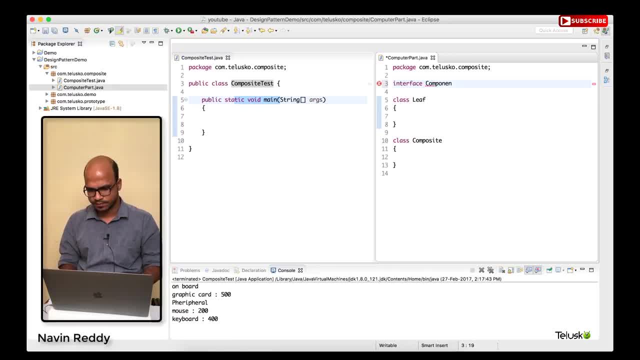 So we will say this is component. So I am creating an interface called as component. Inside this interface I want. so both these classes need to have a common method Which is public void showPrice. Because I am focused, I am more concerned about the price here. 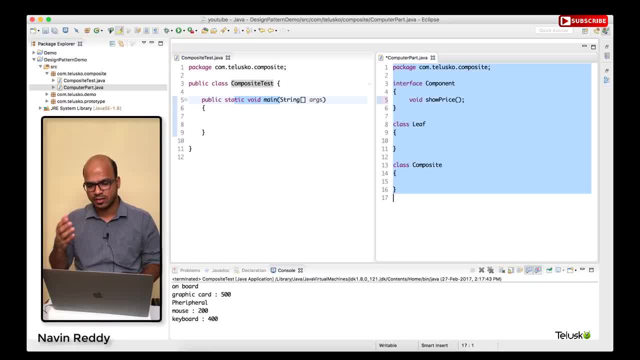 In fact, when we talk about the interface, we don't have to create, we don't have to assign the modifier there. Both these classes, leaf and composite, need to implement that interface. We will say implements. We will say implements component. Oh, not compatible, it's component. 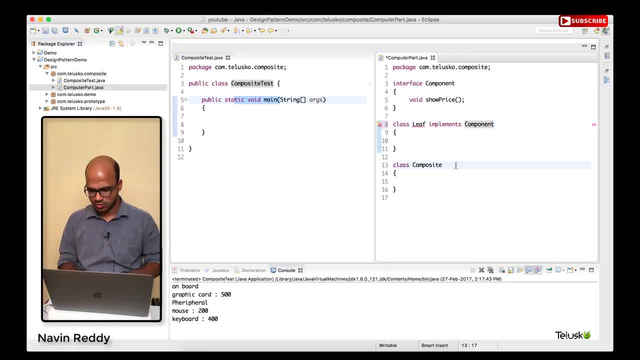 It's typo there, Okay. and then same goes here. We will say: implements component. So what we have here is we have two classes: leaf and composite. Both are implementing show method. Now just to, it is compulsory for us to define that method, right. 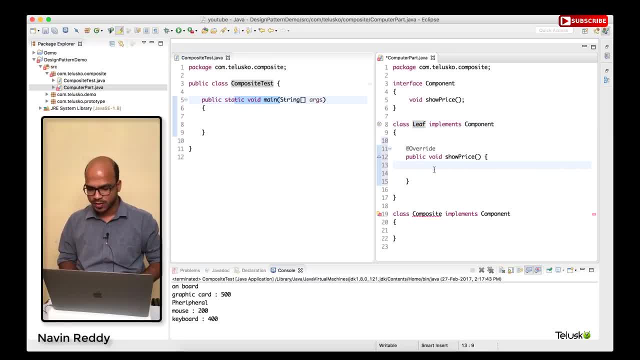 So I will say: define the method. I am not going to specify anything now. And the same thing is applicable for this one. I am saying: composite, implement the show method, And that's done. But then when I say composite, So composite will have list of objects, right. 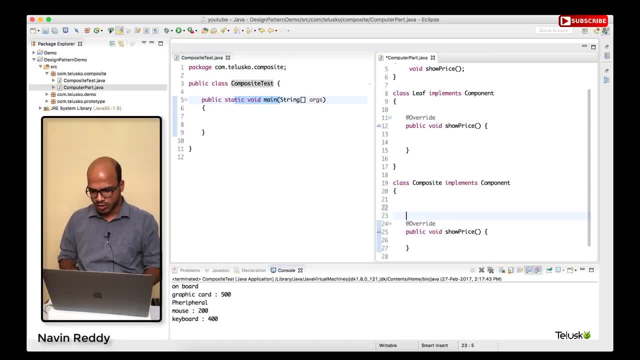 So it will have list of components. So what I will do here is I will say list of component, Because of course when you say you are going for so one composite object will have lots of component. Now again, when you say one composite object, it can have a leaf object or a composite object, right? 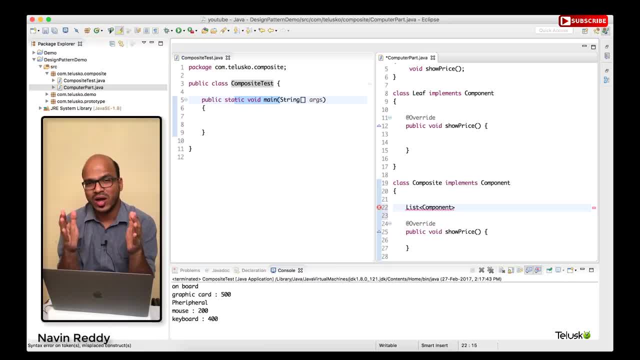 Example, when you talk about a cabinet. Now a cabinet is a composite object. Now, inside a cabinet we have motherboard, which is itself a composite object, And then we have a hard drive, which is a leaf node right. So we will say list of component. 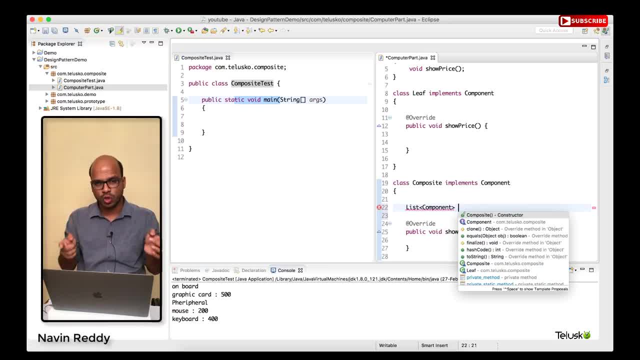 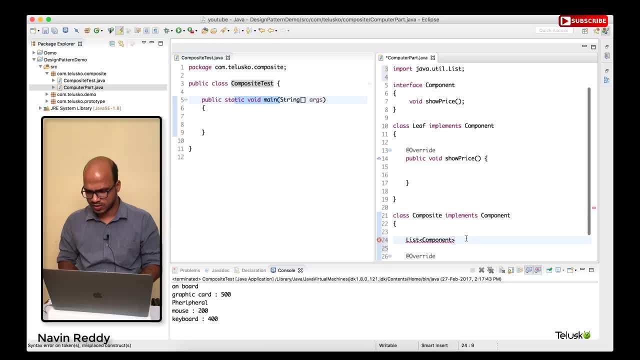 Because a composite and a leaf node- both will be supported by component, right. So I will say this is list. Okay, I have imported the package. Yes, Let's do that. Okay. Then we will say components. We will say components, Okay. 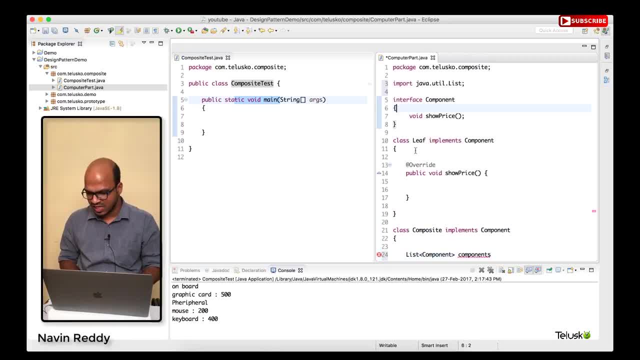 Then watch. In fact, I forgot one more thing: Both this leaf and the composite should have a variable which is int price, Because we need a price there, right, And in fact in every leaf node. I also want a name there, So that we will get the name as well. 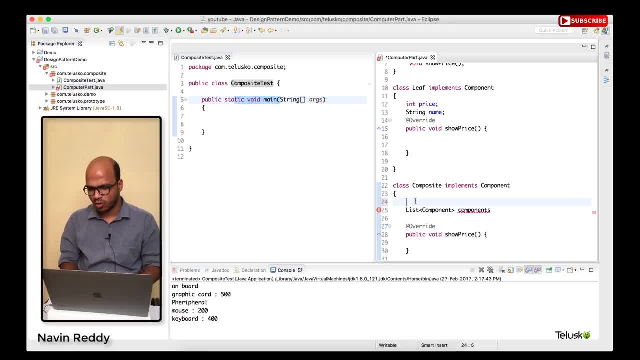 And composite. I don't want price here, I just want name. here We will say name. Let's see what else we need later. Okay, So we have to create components here, right? So I will say new, add a list, Because that's what we want. 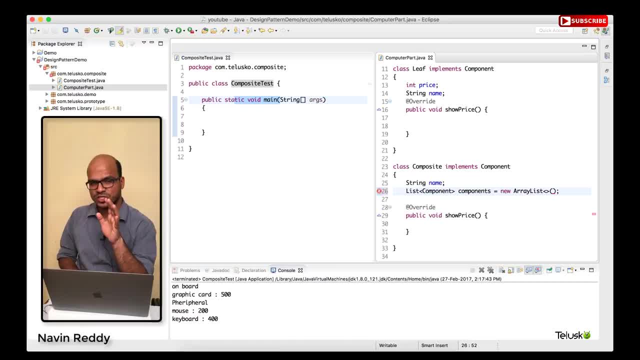 We want to create a list of objects And that's it. We got the add a list here, So this composite should be able to add the component and it should be able to remove the component if you want. But time bin will only say how to add the component. 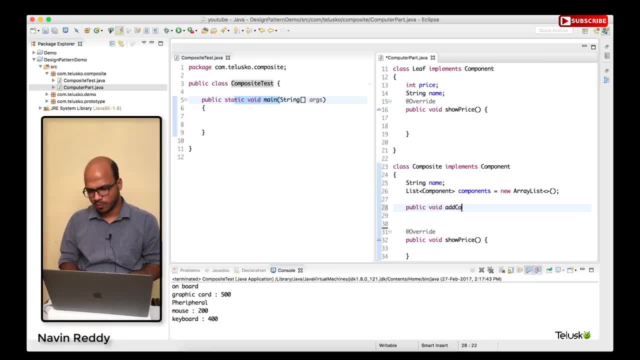 So what I will do, I will say public. I will say public void, add component. which will be able to add the component whichever we want And to add the component. what I will do here is: I will pass an object, I will say component. 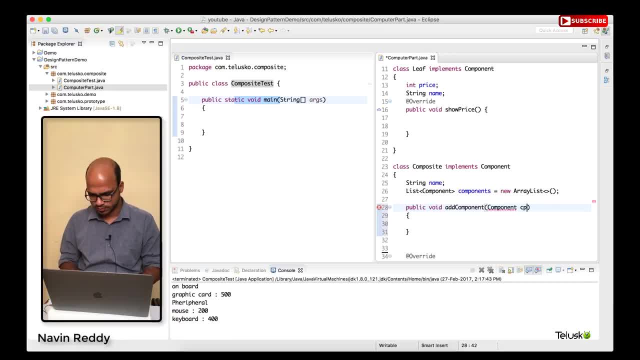 I will say component, comp. We can create any object, doesn't matter. And then in here we will say components, dot add And we will pass the comp object which is com. We have done with our work, Right? So we have, So we are adding the components there. 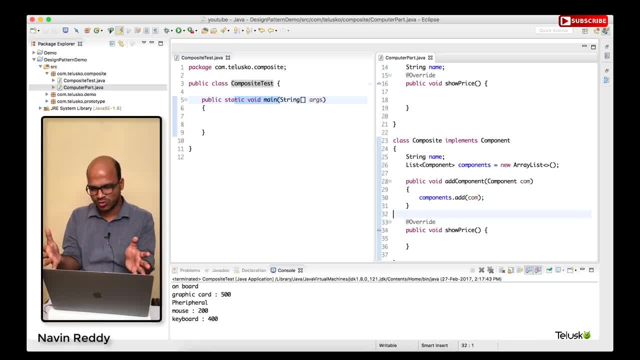 Again, you can use remove method as well, But that's not, Let's not do that here. We can do that later if you want, Okay. And then when I say I want to show the price, Okay, Don't want, Let's not do anything here. 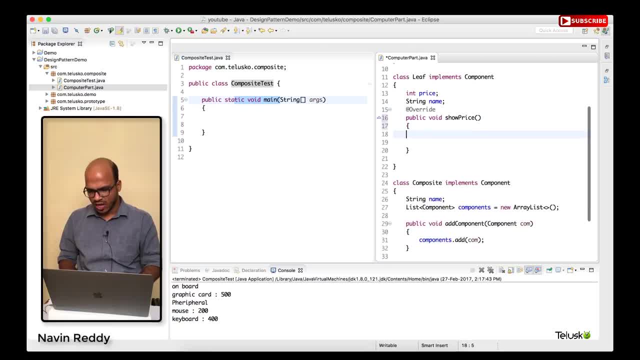 Now, if you go back to our leave, I want to show the price Right. And how do you show the price? It's very simple: We will simply print the price. It's that simple. Right, We are printing the price. 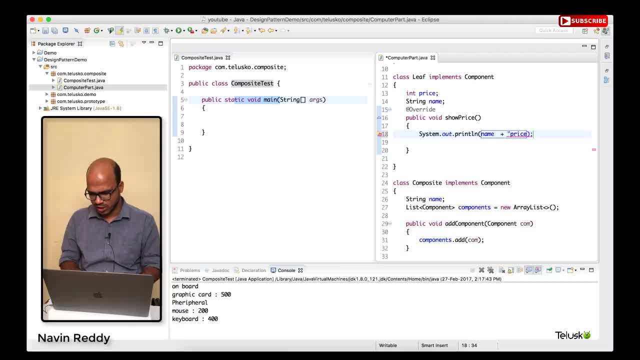 We can also print the name as well. We can say name, colon, In fact name, double quote, What I am doing here. So double quotes, colon and then price. Okay, So I am printing name, then colon and the price, So that it will be printing name and price both. 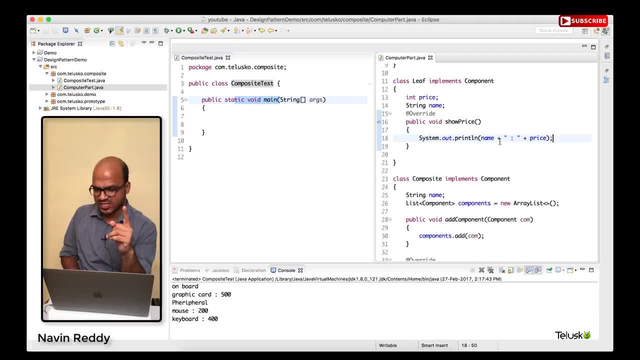 Seems good. Okay, So we got the leave class here, We got the composite class here, And both these classes- leave and component. Composite implements component. Right Now, what else? What else? What else Now when I say I want to show the price, 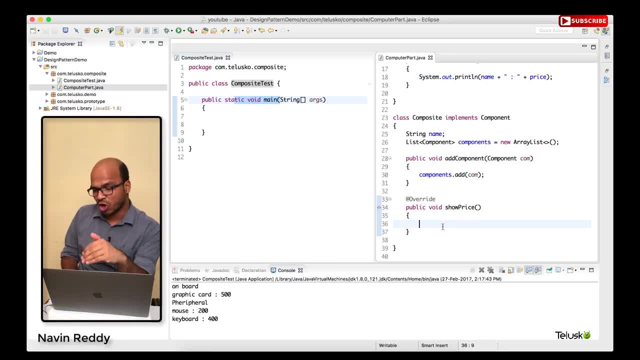 So before printing the price, I want to print the name of the component which I am working with. So I will print System Order Println. So let's say, when I say composite Cabinet, It's one composite object, Peripheral. 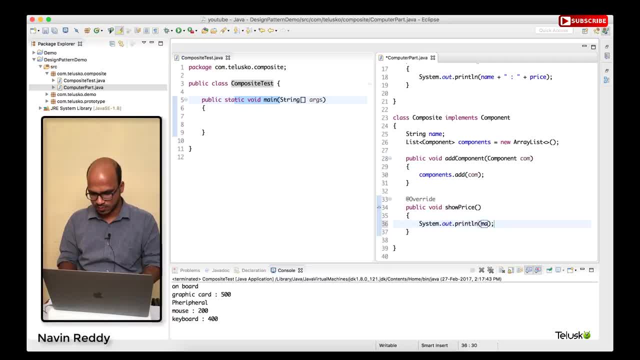 It's one component object. So I will say I want to print the name, So I will print a name here. I am printing the name, In fact, ignore this output. I guess this is what I was doing, some experiment before. So that was the output of that code. 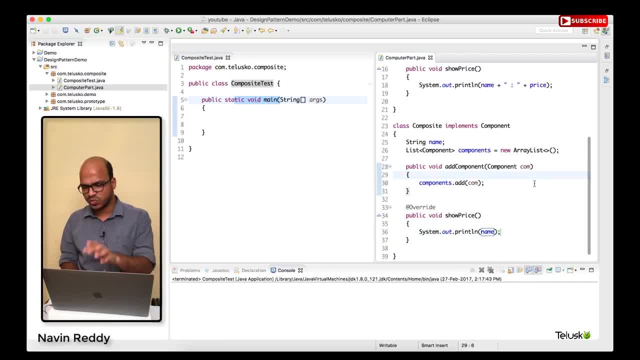 Let's ignore that. And yeah, So once we have this, Once we are printing the name, After printing the name, I also want to print the price of individual component. Right, How do you print the price? So what I will do is: 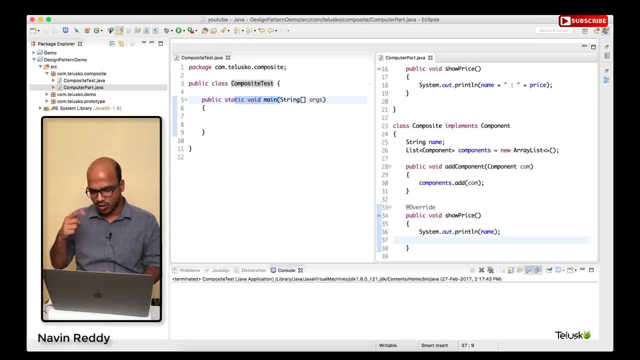 To print the price. Okay, First of all, we have to print the price of the components, Right? So that means we have to iterate To print each component price. We have to iterate Using a for loop, So I will use a for loop here. 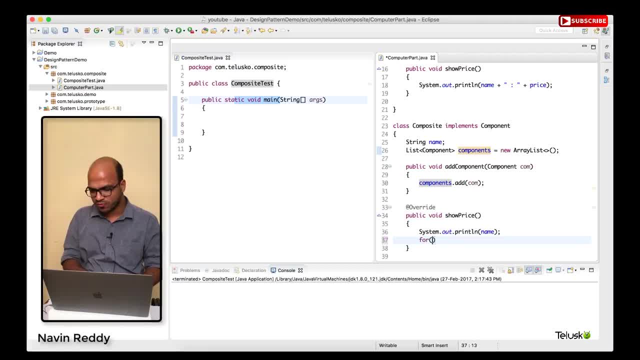 I will say component C, colon. It's components. Again, We can use normal for loop Or we can use announced for loop. That's your choice. Let's print the value now. Now, how can you print the price? It's very simple. 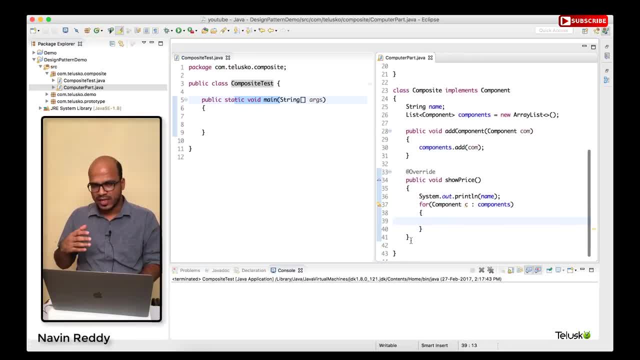 Just simply say C dot Show price. Because when you say C dot Show price, Because when you say C dot Show price, Because when you say C dot Show price, We are So Okay Now. 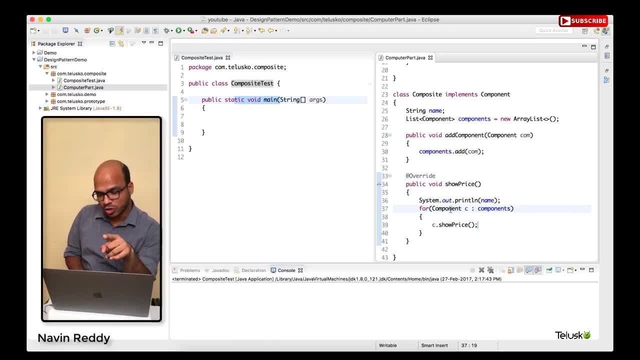 Now this is tricky. Okay Now, since I am not specifying leaf or composite, I am saying component, The component, object, dot, Show price. Now The component which we are getting, Which we are adding in the components, If let's say: 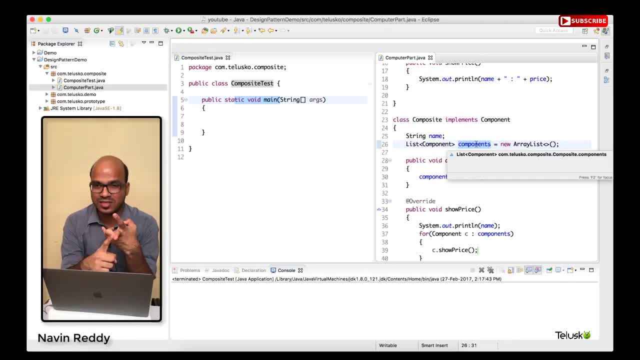 The first component is composite, The second component is composite, The third one is leaf. What will happen for the third one? It is simply print the price Right. So let's say, If you are going for the third component here, Which is actually 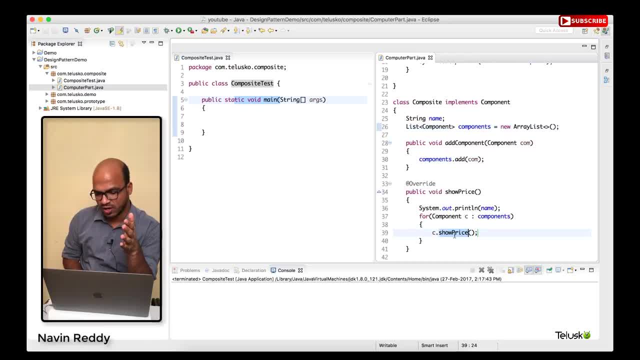 A leaf, Leaf. It will print the price. Right, It will print the price. But let's say The first, one, Second one, Which is your composite. What it will do is For that composite It will again call. 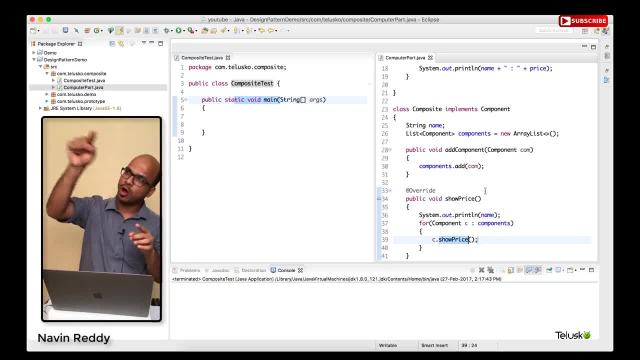 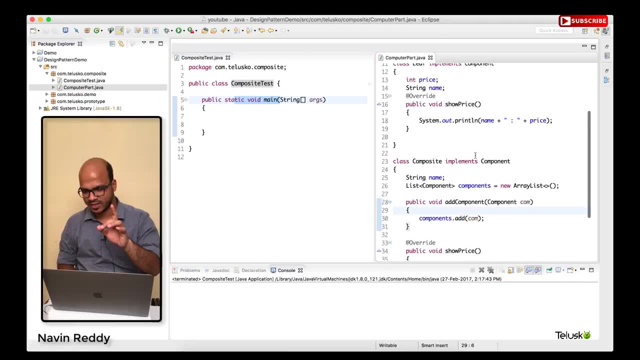 The leaf nodes. So it will go, It will traverse. Okay, From composite Composite Leaf. Okay, Let's do that, Let's, Let's print this So that you will get the Let's. You will, You will get the idea there. 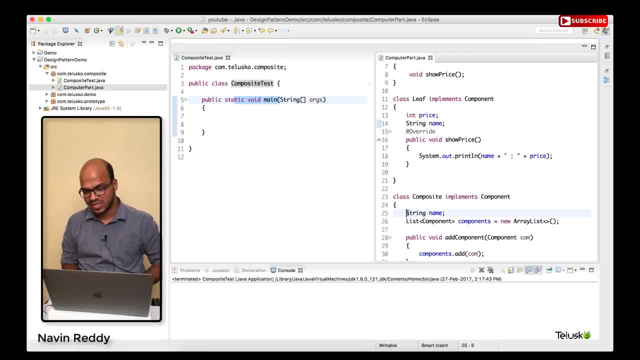 But then We are using these two variables, Right. How do you assign those two? How do you assign these two values, Price and name? So what we will do is I will use A constructor to assign the value. So I will say: 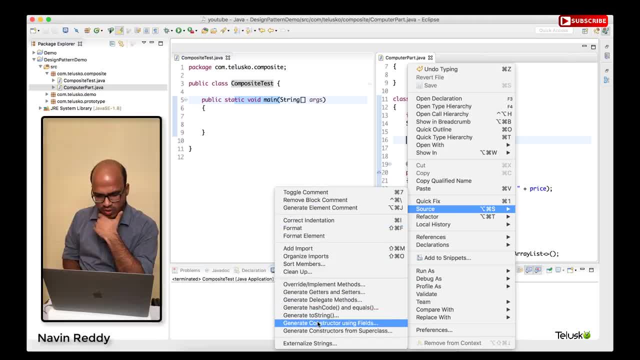 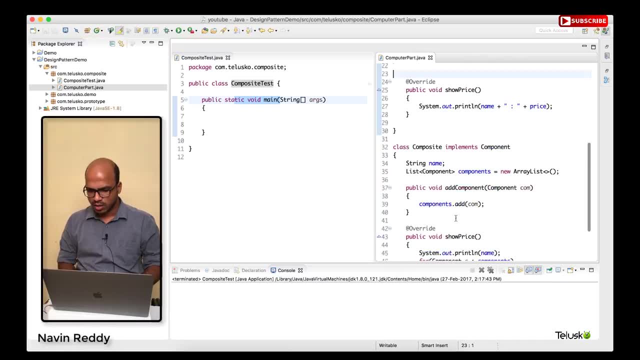 A source And we will say Constructor, Which can take two variables, And we are done with that. Okay, So we have. We have got a constructor Which can take two values And then In the composite as well, To assign this value name. 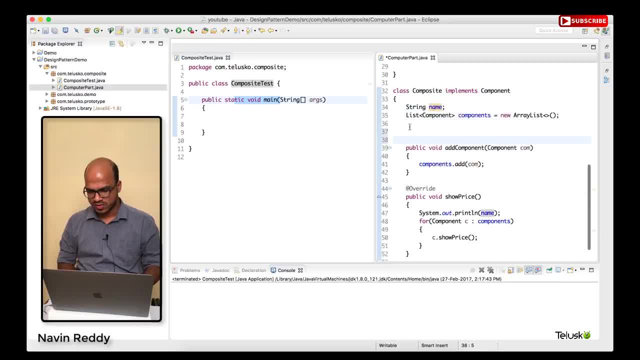 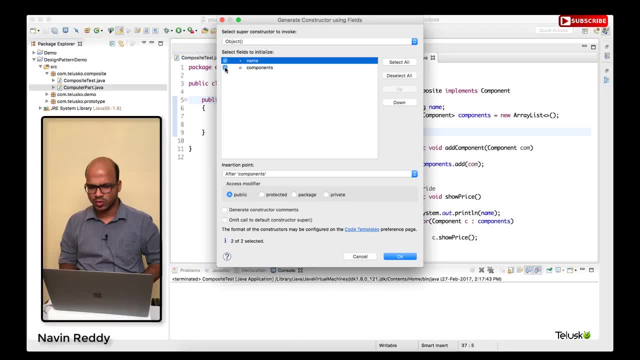 I will use a constructor, So I will say: Write like And we will say: Source: Constructor. Okay, With With With name. No, I don't need components there, Just name. Okay, So how I am doing that. 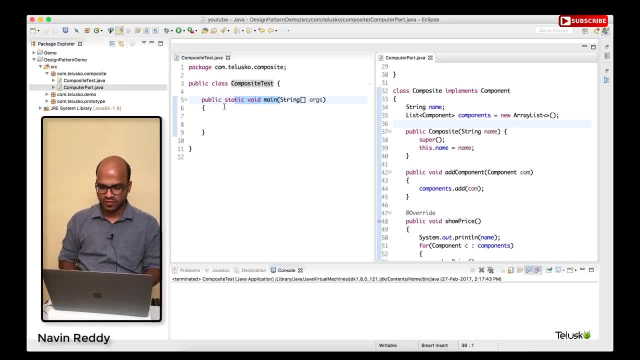 Because When I want to create the object, I can assign the value there itself. Let's start with the first one. Now, when you say Let's, Let's create this hierarchy, We have a computer. Computer will have Two parts. 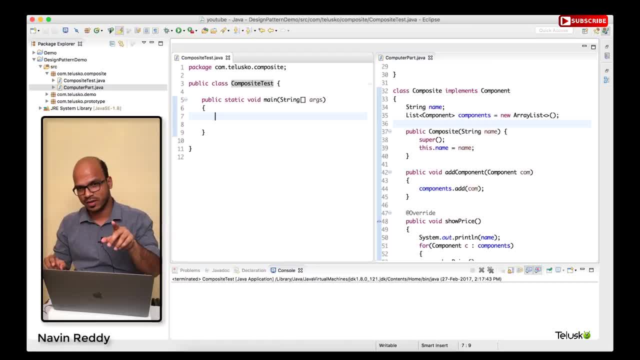 Cabinet And peripheral. Cabinet will have Hard drive And Motherboard, Peripheral will have Keyboard Mouse. We will not create all the objects. Let's go for one or two. So let's create the first one. I want a leaf. 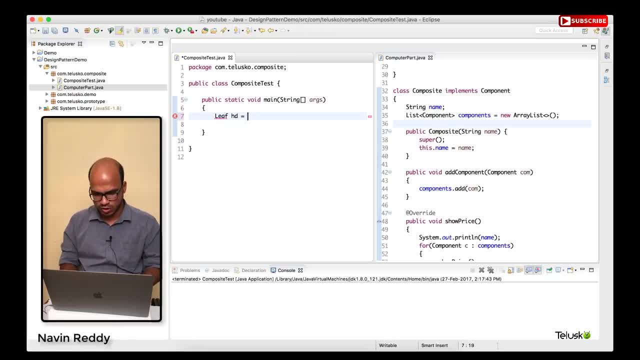 I will say Leaf Motherboard. Motherboard is not a leaf. We will say Hard drive Package. I guess Is it the problem. Okay, Let's import the package. No need, Because they are the same package now. 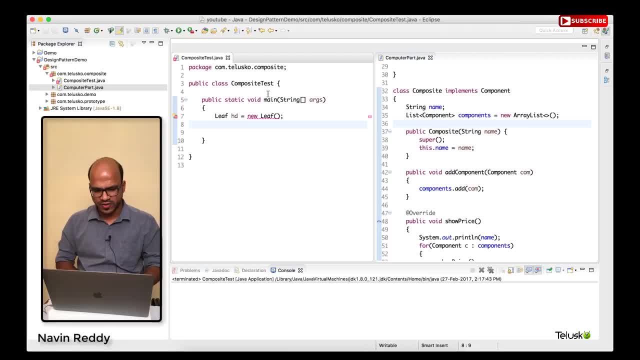 We will say New Leaf, So we got our first component. In fact, Instead of saying Leaf, I would also say Component. Right And anyway, They all are component, So it doesn't matter. So we will say: 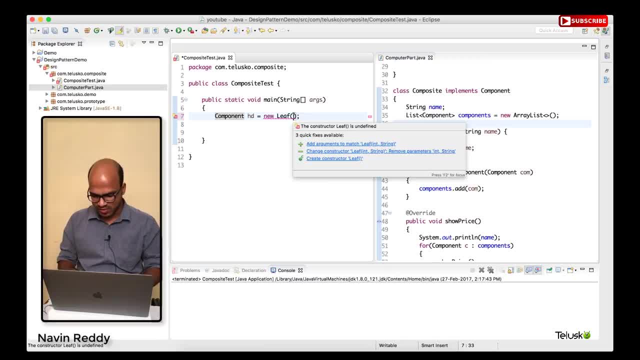 Component: Ht equal to new leaf. Now, While creating this leaf, I will I have to specify The parameters Right. So I will say the name Is Price. Again, I am going for rupees here, Okay, 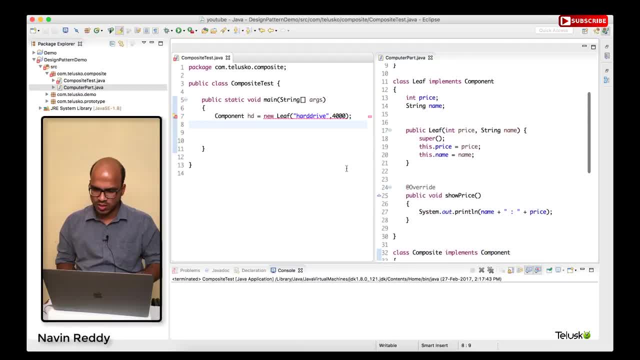 And we are getting an error Because I guess I am missing the sequence here. The sequence is: Oh, It's price And then the name. So we will cut this part, I will say Comma And we will set the. 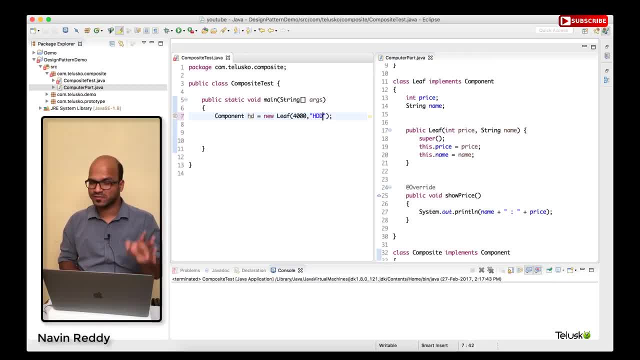 Name there, Oh, Okay. So we will say This is: Oh, Let's say Let's, Let's, Let's say Hdd. Okay, Instead of saying the entire thing, And let's name it as A mouse. 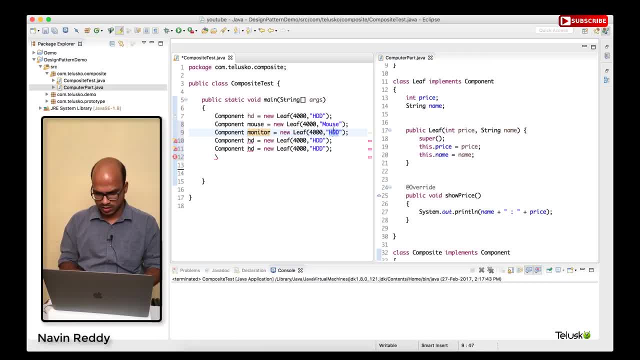 And then we got A monitor And let's say This is A monitor, And then Let's go for Motherboard, But then motherboard is not a leaf, Right? So I will say: A ram And that's your. 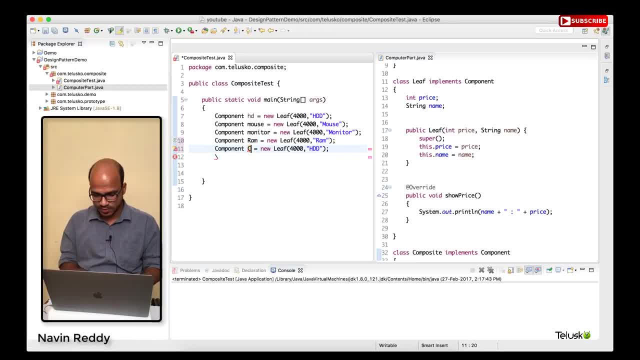 Ram, And then we need one more Which is, Let's say, CPU, And that's your CPU. So we got this four leaf object Or five leaf object. Now, once you got the leaf object, What we need Here is the composite objects. 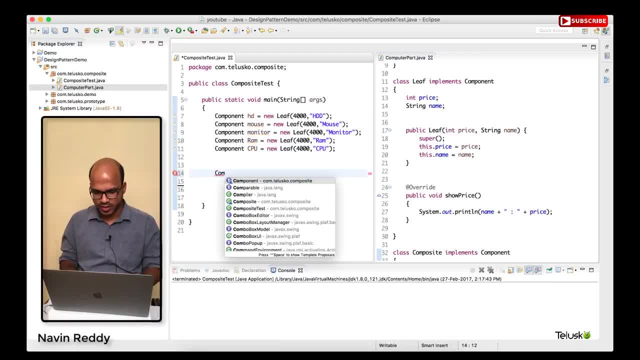 Right, So we will say Component. again, This is component, Right, So we will say Component. And this time we will go for peripheral. We will say Ph, Equal to Neo. We will say Composite. Am I missing spelling here? 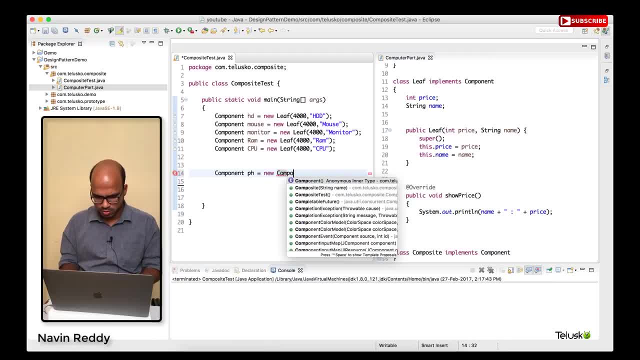 We will say Composite- What's that? Yeah, Composite. And then we have to pass a name, Right? We will say: This is Peripheral, Just ignore this spelling. there I will say Perry, Because I am very bad with. 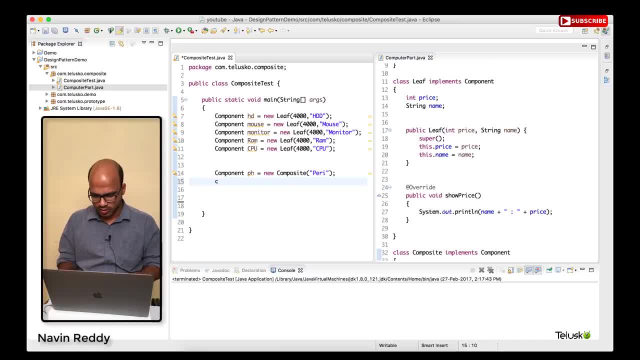 Spellings here. So we will say Perry, We will say Component, We need one more component here. In fact We need three. One is peripheral, Then we have What else? Cabinet? And then we add: We will add one more. 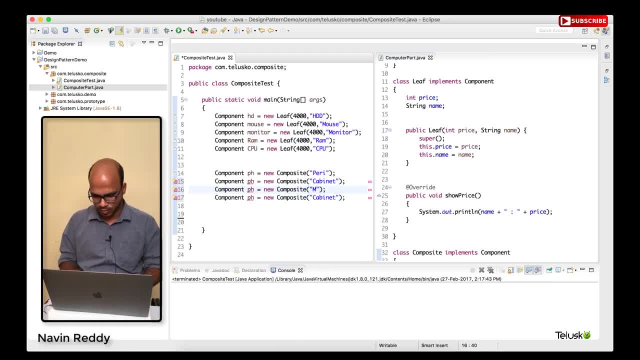 In fact We need two more. One is motherboard. We will say M, motherboard, MB, And then we have Computer Right, Because ultimately we need a computer Right, And then this would be Cabinet Right, And then this would be: 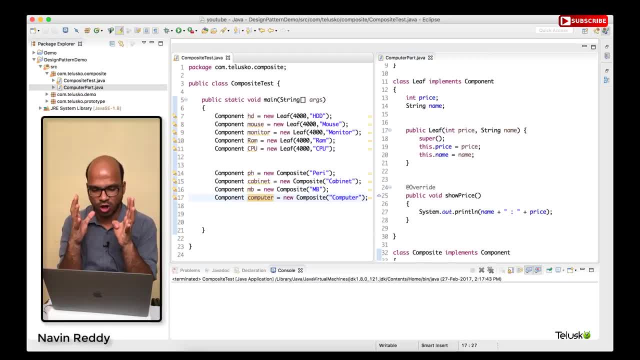 Motherboard, MB, And this would be a computer. So we have Five objects And then, Once we got Five components, Once we got Five- Name here I mean Five Composite objects- Let's add this composite object. 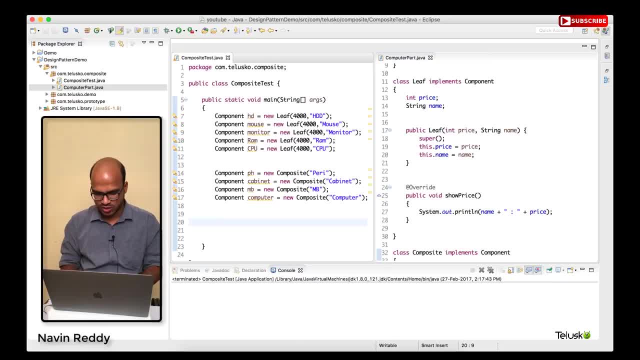 Right Now, how do we add this composite object? It's very simple: In peripheral devices We have, So We have to add HD here. So we will say PH, Add component. Oh, Unfortunately I don't have add component inside. 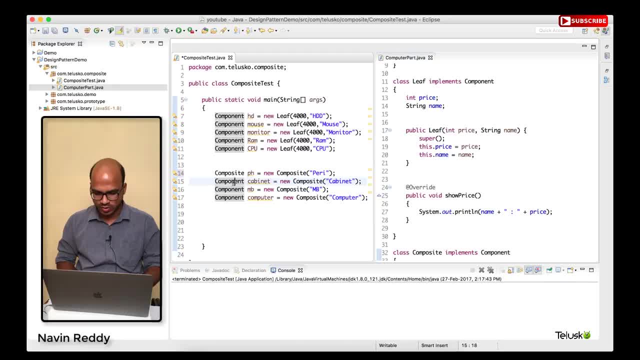 That method. So what I will do, I will go for composite here, Just to be on safe side. Set the method, Components Composite. So what I can do, I can say PH, Add component, And we can In peripheral. 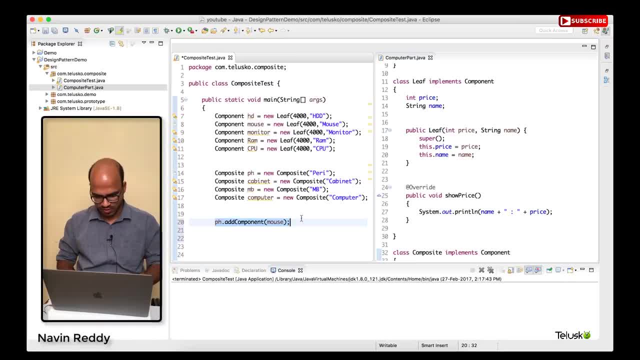 I want to add Mouse, So I will say Mouse, And in peripheral I will add What Monitor? Which is Monitor Then? So we got the peripheral there, Let's go for cabinet now. So we will say: 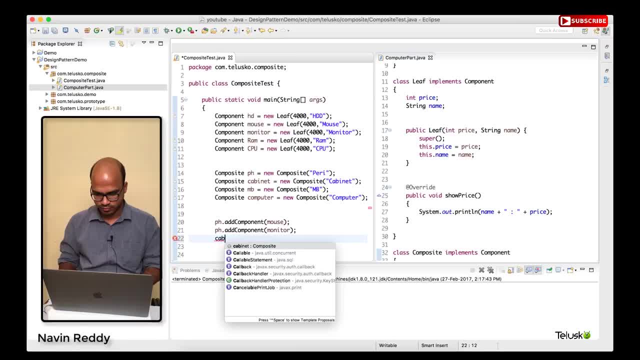 Inside the cabinet. What we need is We will say Cabinet Dot, Add component And this would be Inside cabinet, Inside cabinet. We will be having A hard drive, We will say HD And we will Inside cabinet. 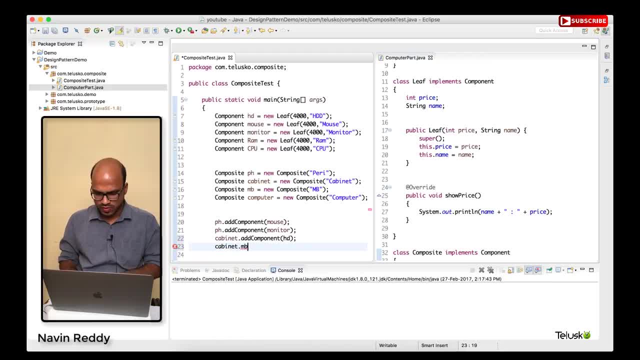 We will be also having motherboard, But then we have not created the object yet. We have created the object for motherboard. So we will say Add component And we will say MB. Now, once we have added the peripheral And the cabinet, 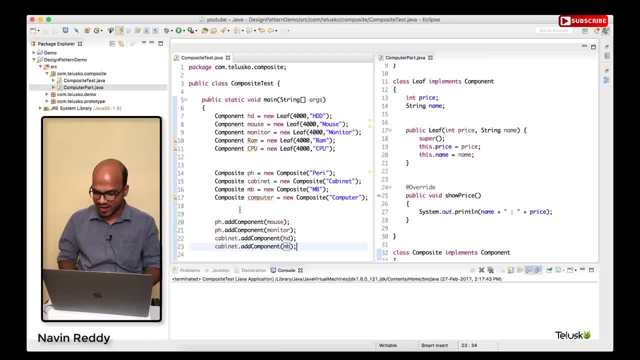 But inside motherboard We have two things Right: We have RAM and CPU. So we have to do that as well. So first we have to add into motherboard. We will say Add dot, I mean MB, Add component, And we will say: 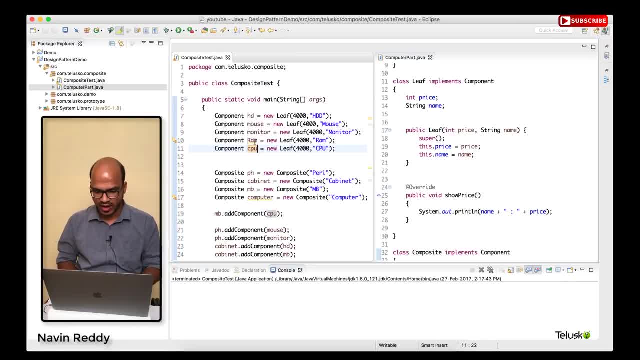 RAM. So we are adding RAM, We are adding CPU and RAM in motherboard, Then we are adding Motherboard and hard drive Inside cabinet And then we are adding Mouse monitor Inside peripheral Right. We are adding, We are adding. 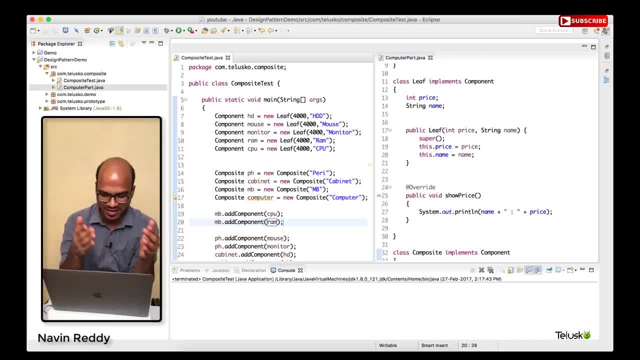 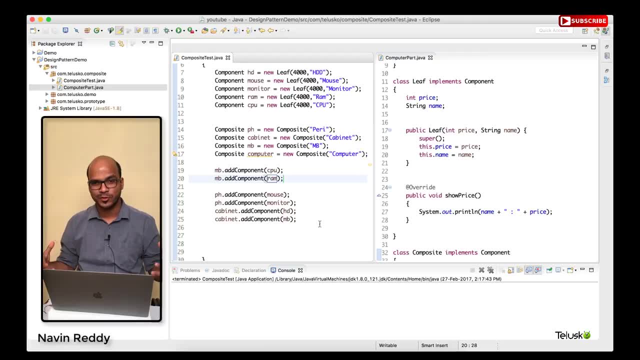 Lots of components And I can feel now I am actually building a computer here. I am assembling a computer And then we have to add Peripheral And the cabinet Inside your Computer Right, So We will say Computer. 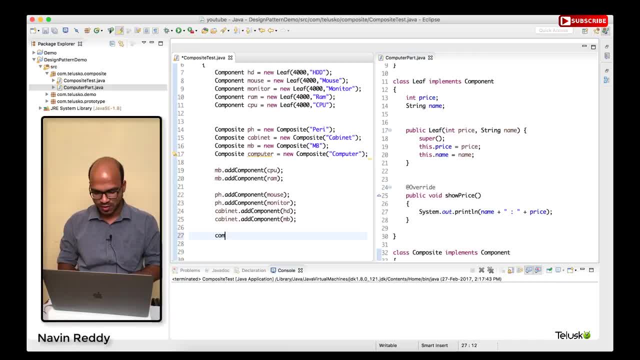 And then we have to add Peripheral And the cabinet Inside your Computer, Which is Computer, Which is computer here, And then say: Add component. We have to add two things: One is PH, Which is peripheral, And then we have to add: 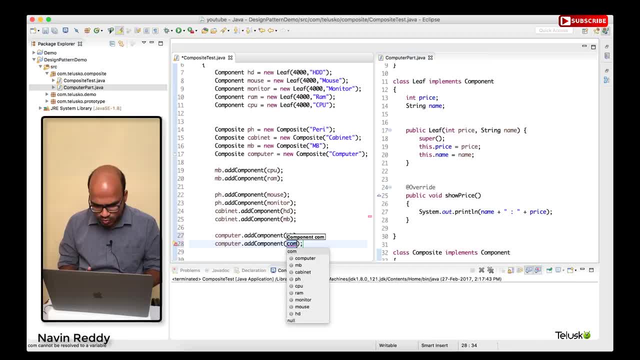 We will say: Computer Dot, Add component. We have to add What we have done. We have done with the Okay, Hold on. So we have added the Peripheral. Let's also add the cabinet. So you can see the hierarchy here. 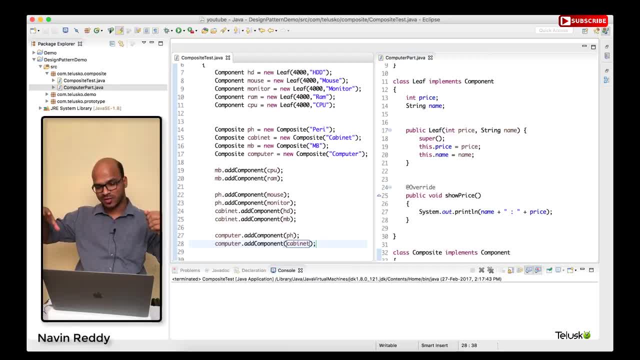 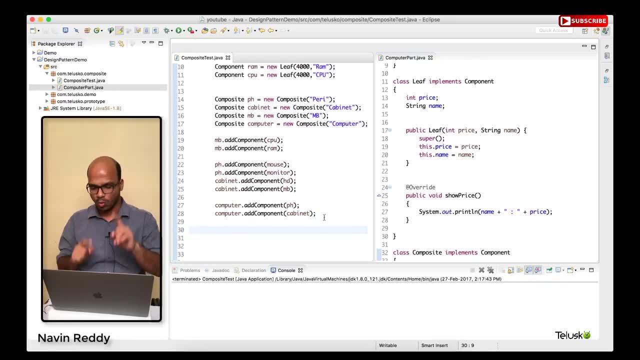 Right, So Inside motherboard We have peripheral And we have cabinet Inside cabinet. Okay, Code. And ultimately, If I say, If I want to print only one, So Just to, Just to show you demonstration, I will print. 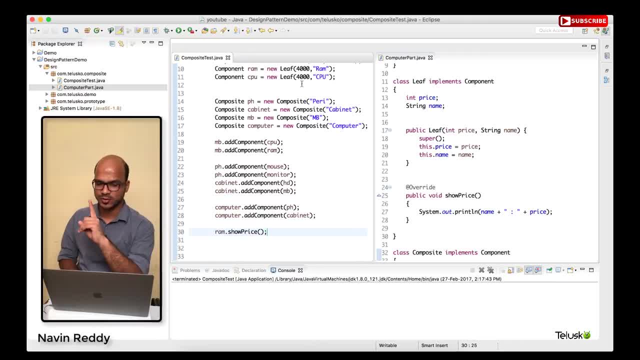 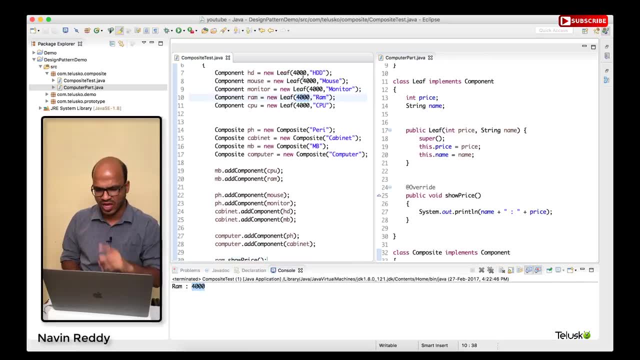 The Price of RAM. I will say RAM dot Show price. Just one price. Okay, If I run this code You can see it is printing only RAM price, Which is 4000.. Is it 4000 RAM price? 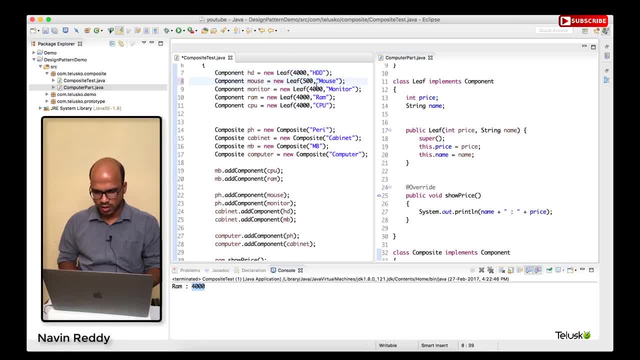 Yes, We have setting it 4000.. Oh, We have all the same price here. Let's say, Mouse is 500.. Monitor is, Let's say, 8000.. And then we go for CPU, Which is 9000.. 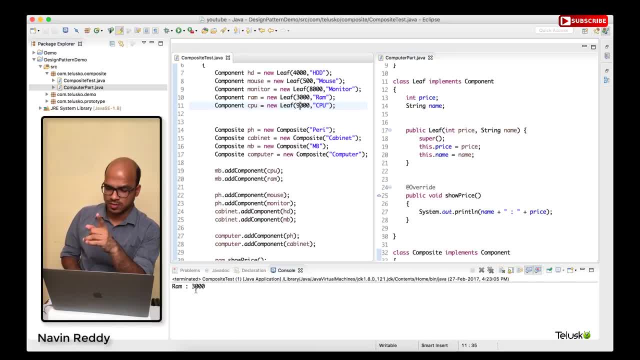 Just to have a different values there. You can see, for RAM We got 3000.. But the moment I say I don't want the price of RAM, I want to, I want the price of entire peripheral, I will say: 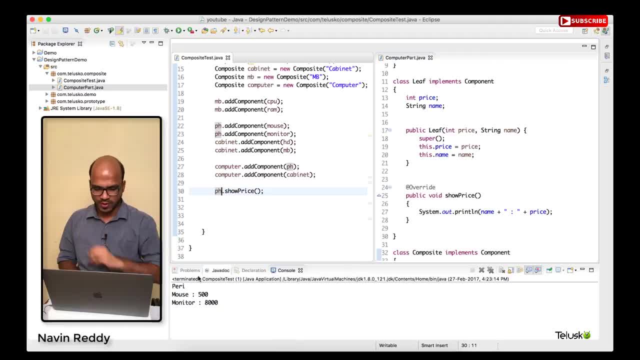 PH dot Show price. So You can see I got peripheral And I am also printing the value. So Inside peripheral We have mouse and monitor Which cost 500 and 8000.. So The amazing thing about composite is: 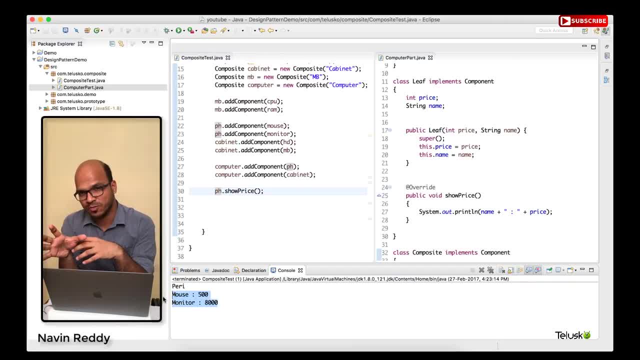 You can use the same operation On leaf object Or even composite object. If it is leaf object, It will print the value. If this composite object, It will print all the values Of the leaf objects. Now Amazing thing is: 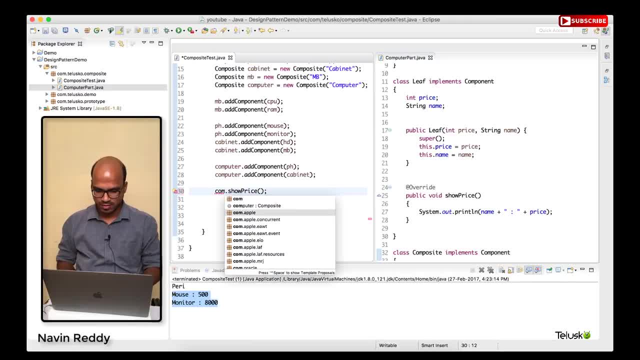 If I say Computer here, Which is the top of the hierarchy, If I say Computer dot, Show price, You can see It will print everything. It will print First of all. It will print computer Inside computer. We have peripheral. 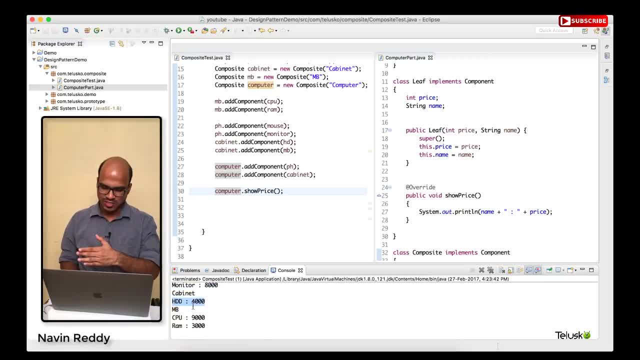 Peripheral- is printing These two objects, And then cabinet is printing The cabinet values, Which is MB, And motherboard, Which is a part of cabinet, And then it is printing that as well. It's so awesome, Right? So that is. 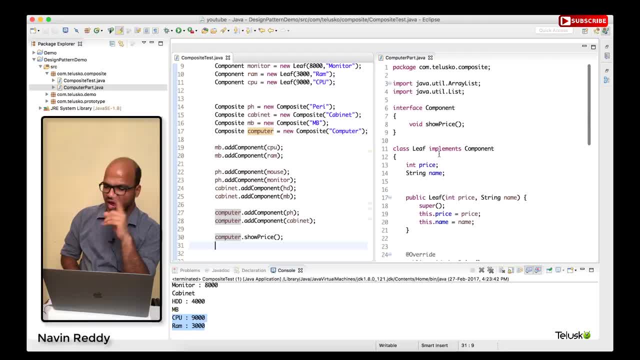 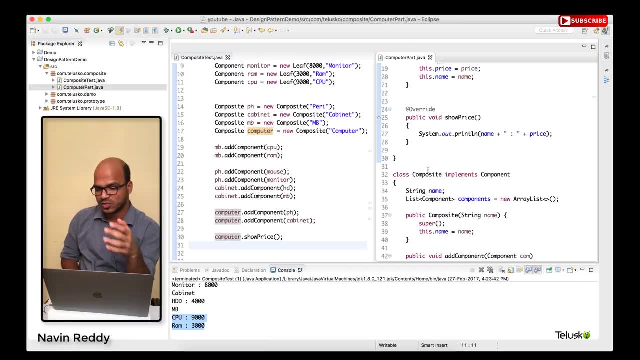 That is how your composite design pattern works. So We have Glimpse, We have, We have an interface Which is component, And then we have two classes Leaf And we have composite. Both are implementing components, So that we have 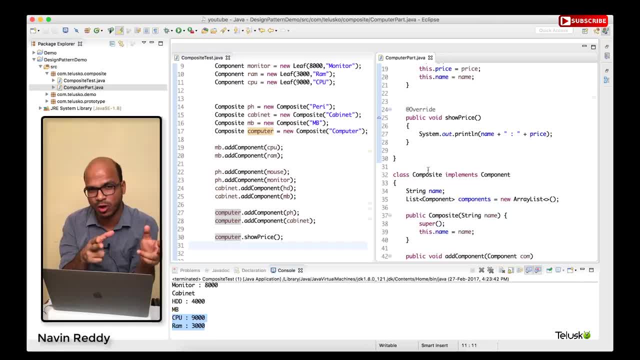 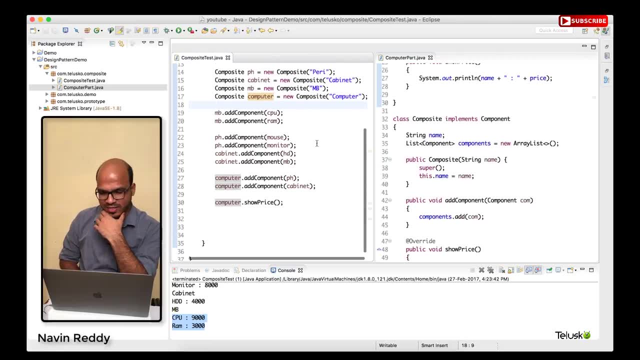 Some common thing in between, Because whatever operation You want to perform On the leaf object, The same operation Should be Need to be performed On the composite object, Right? So Yeah, That's how it works. We have done.